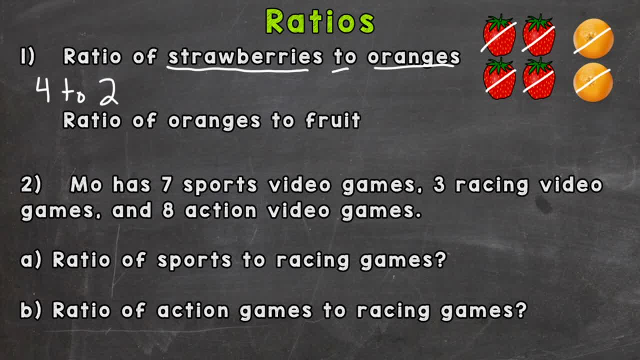 we can write a ratio out. We can also use a colon. So we could say four colon two, and that just means four strawberries to two oranges. Or we can use a fraction: four to two. Whatever comes first is your numerator, the top number. Whatever comes second, your denominator. 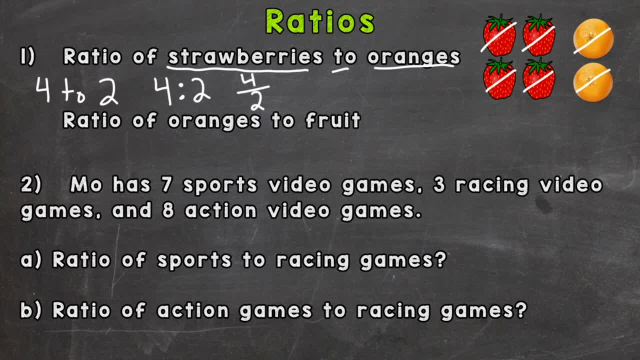 Now, with ratios, just like fractions, you always want to simplify. if it applies to that ratio, And four to two, we can simplify. We need to find the greatest common factor between four and two. So what can divide into both four and two? Well, we can divide them both by two. 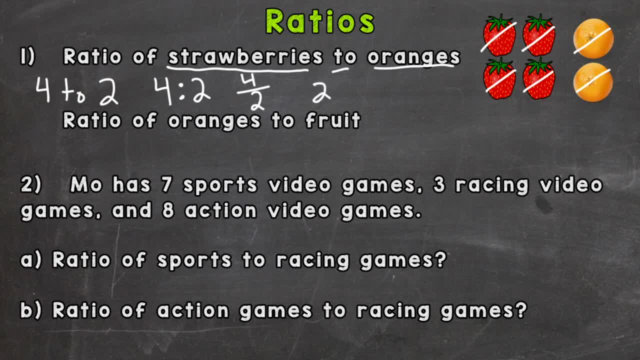 So three divided by three, So three divided by three equals plus two. So three divided by three equals two. So three divided by three equals two. So three divided by three equals two. So 4 divided by 2 is 2, and 2 divided by 2 is 1.. 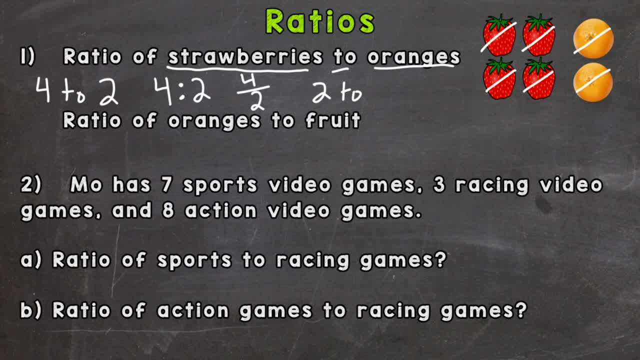 So I'm going to rewrite the simplified ratios 2 to 1.. Next I'll write it with the colon: so 2 to 1, 2 strawberries to every 1 orange, And then, lastly, fraction 2 to 1.. 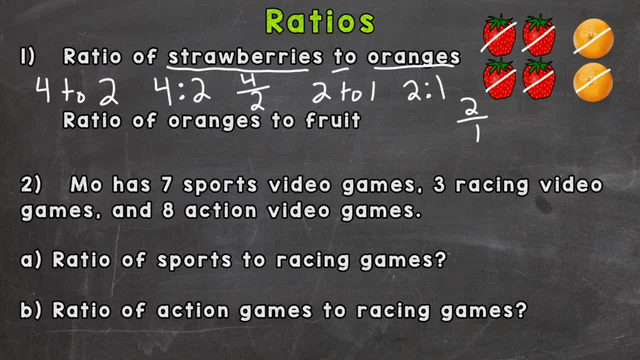 And let's take a look at the picture up at the top right And, as we can see, 2 strawberries to 1 orange, 2 strawberries to every 1 orange. So our simplified ratio matches our picture. Let's take a look at the second part of number 1, the ratio of oranges to the total amount. 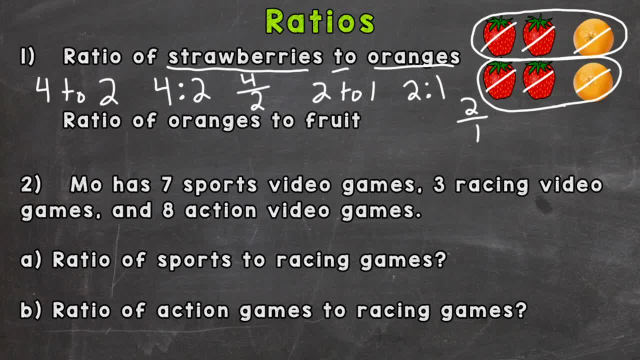 of fruit. This is called a part-to-whole ratio because we're taking a part of the group, the oranges, to the whole group of fruit. So, oranges, how many do we have? Well, 2, I'm going to use the colon for this. 2 to how many total pieces of fruit? 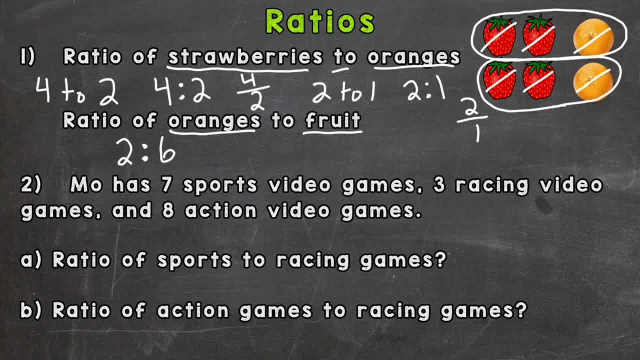 Well, 6,, 2,, 2,, I'm sorry, 2 oranges to 6 pieces of fruit. Now, this one can be simplified, because there's a greatest common factor between 2 and 6.. We can divide them both by 2.. 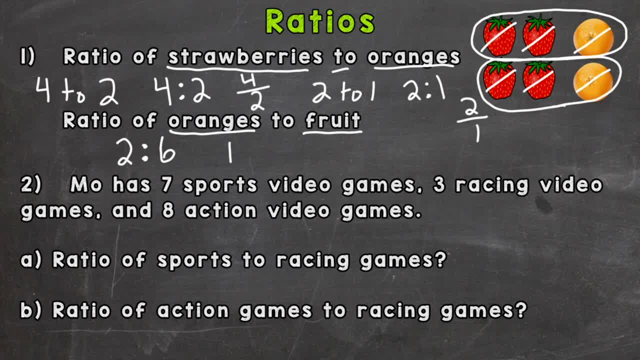 And 2 divided by 2 is 1.. 2 divided by 2 is 1.. 2 divided by 2 is 1.. And 6 divided by 2 is 3.. So the simplified version is 1 orange to every 3 pieces of fruit. 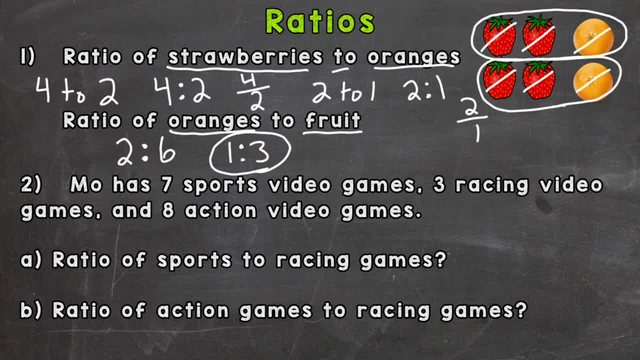 So again, that's a part-to-whole ratio. Now the first part of number 1 up here. this was part-to-part because the strawberries are a part of the group and we compared it to the oranges, which is another part of the. 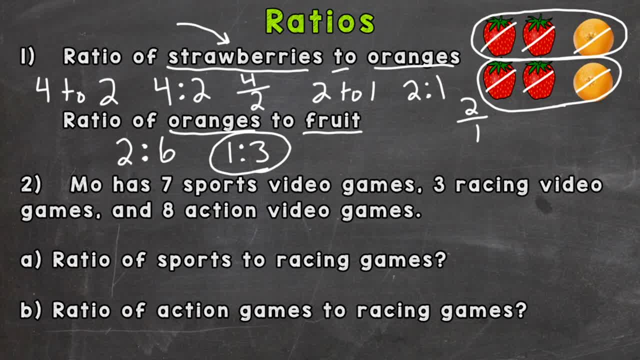 group. All right, Let's take a look at number 2.. Mo has 7 sports video games: 3 racing video games and 8 action video games. So we're given the situation in words here, without a picture, And we need to find the ratio of sports to racing games and then the ratio of action. 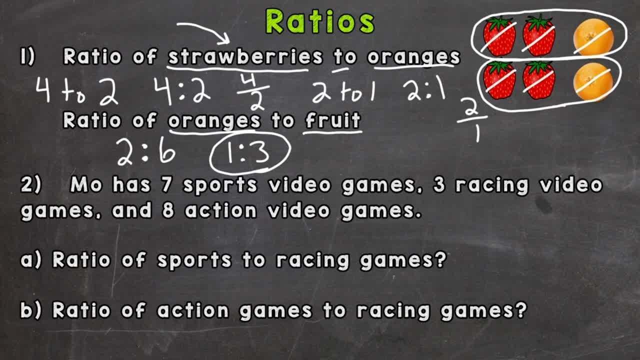 games to racing games. So let's do a first here. And we need sports first to racing games. So, how many sports games? Well, 7.. And I'll use the colon again. And we are now finding how many racing games. 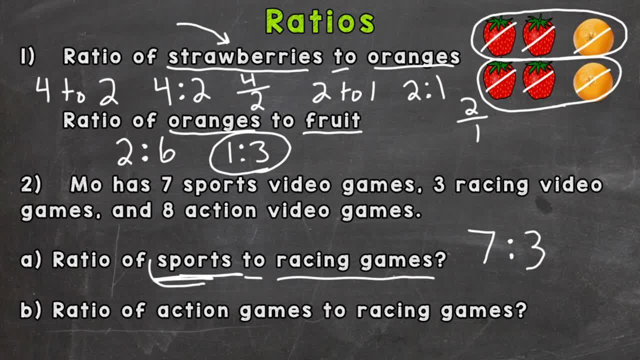 Well, 3.. Sports needed to come first because it's first in our situation. Racing comes second because it's second in our situation. So there are 7 sports games to every 3 racing games. That one is in simplest form already. so we're done. Let's take a look at B: Ratio of action. 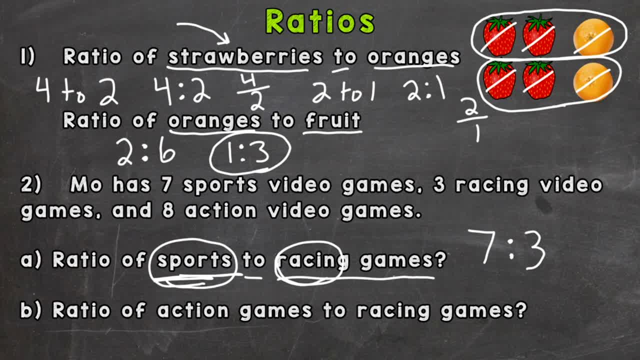 games to racing games. Well, how many action games? There are eight action games- That needs to come first because it was first in our situation- And two racing games And there are three racing games. So there are eight action games to every three racing games. That one is in simplest form already. 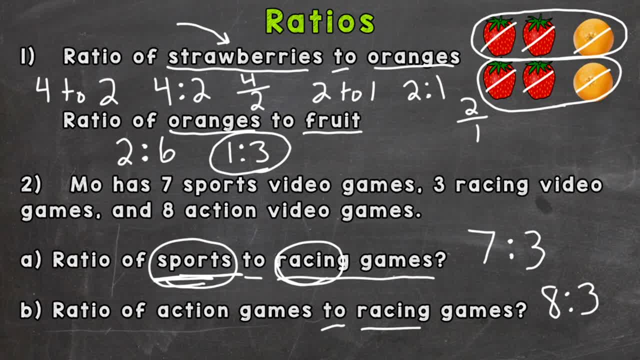 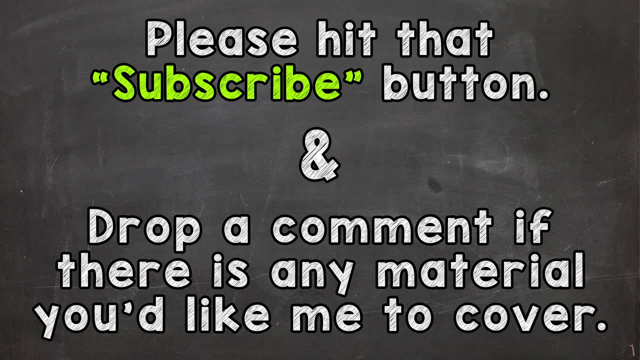 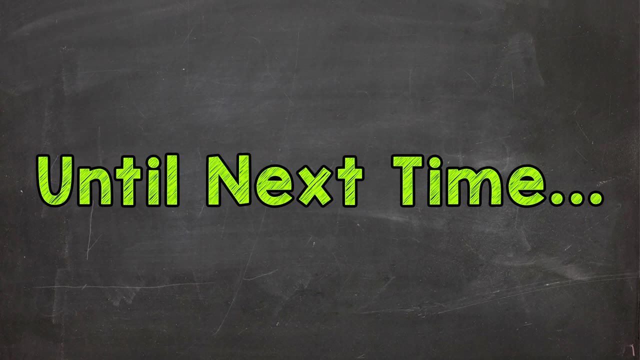 just like part A. So we are done with number two there. So there you have it. There's how we write out ratios for different types of situations. Hopefully that helped. Thanks so much for watching. Until next time. peace Captions by GetTranscribedcom.